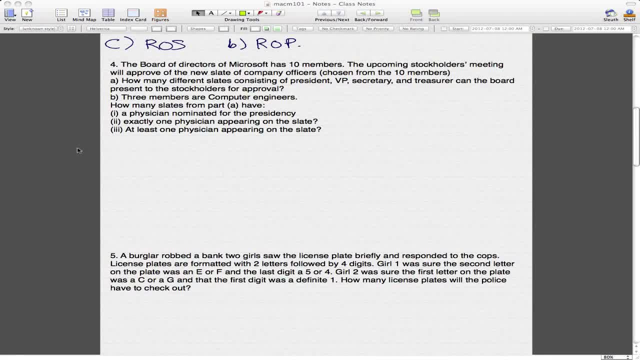 Right. so I hope you guys actually did the exercises or examples, because they're actually really worthwhile and you need to do a shitload of examples and exercises in order to ace a course like, or even pass a course like, discrete math, So I really hope you did them. 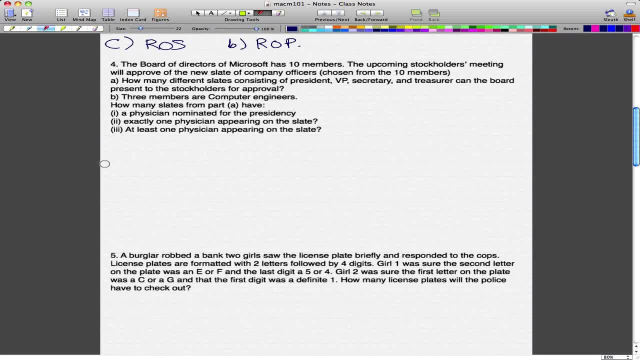 So the board of directors of Microsoft has 10 members Now. the upcoming stockholders meeting will approve of the new slate of company officers, which is chosen from the 10 members. So here's A. A is: how many different slates consisting of president, VP, secretary and treasurer can the board present to the stockholders for approval? 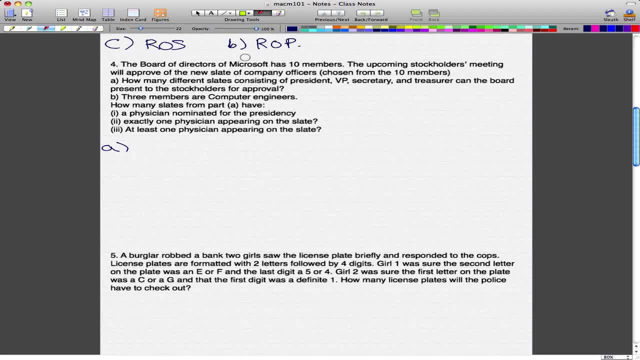 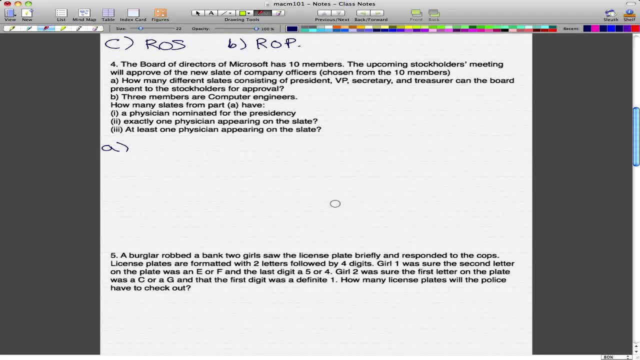 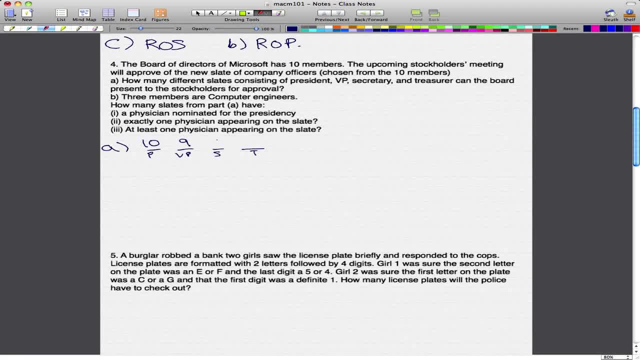 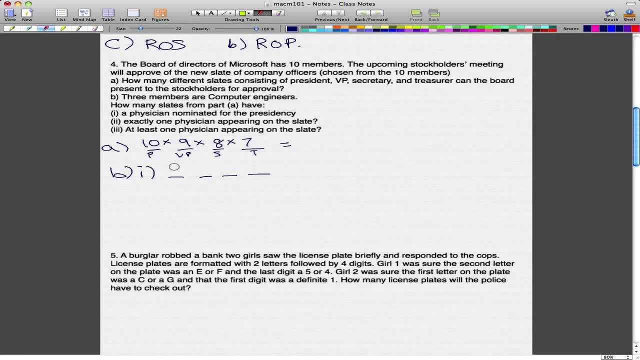 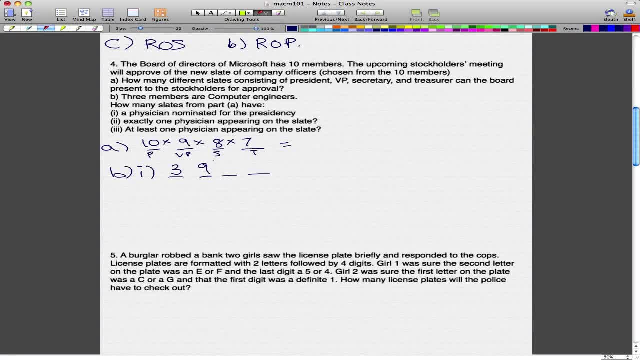 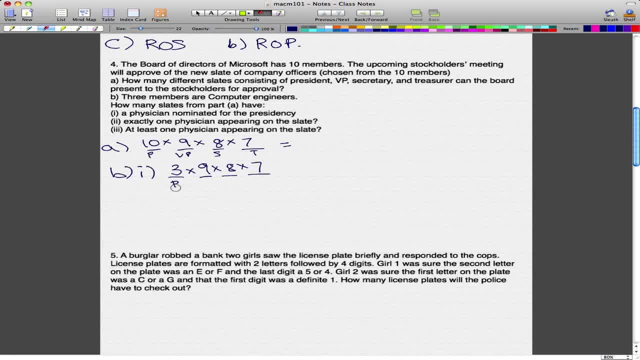 a computer engineer that takes the president role, all the other roles or all the other, all the other members that are not computer engineers. they cannot take the president presidency role because it sees a physician nominated for the president. we have three members that are computer engineers. I don't know. 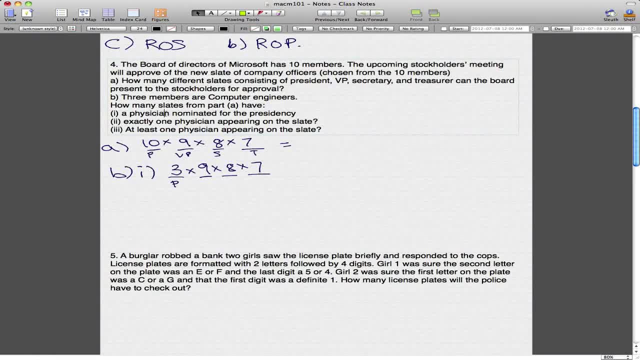 why that's his position. probably because I modified this example from the book, so let's just change this on the fly. so yeah, so that's the reason why we have three for presidency, because there are only three members that are president. so I don't know why that's his position. probably because I modified this example from the book, so let's just change this example from the book. so 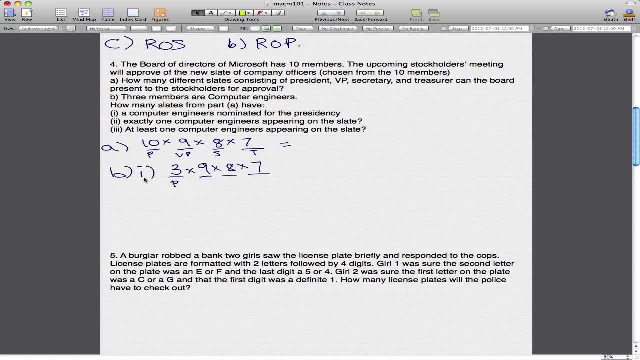 let's just change this on the fly. so let's just change this on the fly. so all the other members that cannot take the presidency role, they cannot have the presidency. we have three choices for presidency, but then the other engineers are not out of the choice. the other two engineers can take other roles. So then we just go back to. 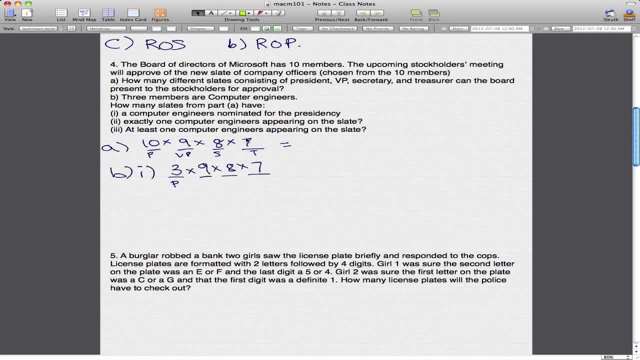 our normal calculations and after picking one person for for presidency from the commuter engineers, there are still nine people: the two engineers and the seven other members that are not engineers that can be chosen for VP. So we have nine for VP, and then we pick one of the nine for VP. then we have eight people. 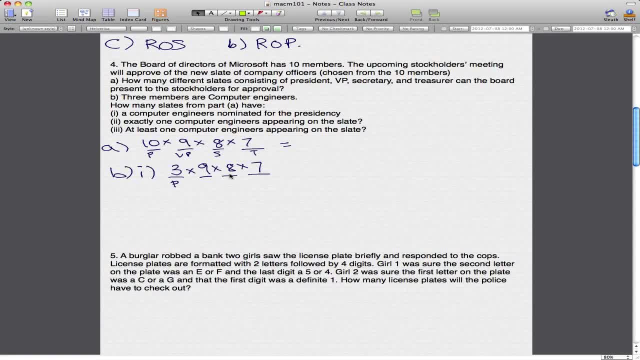 pick one of the eight members for secretary and then we have seven people and we pick one of the seven for treasurer, And it's as simple as that. I know that I haven't. I don't think I explained that well, but I hope you guys get it. 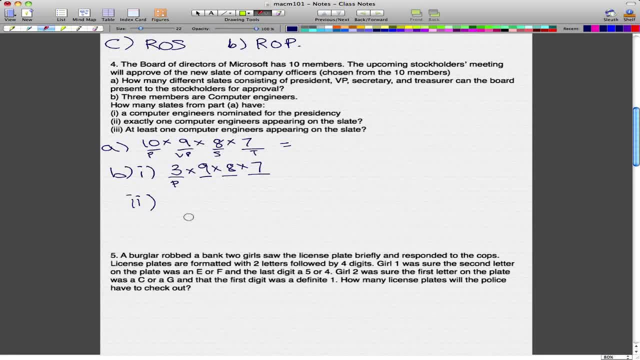 So for the second one is exactly one. computer engineers have to be on the slate, So this one, this one is simple as well. So pretty much, a computer engineer has to be on the slate, exactly one. So for this is one case in which the computer engineer can appear. 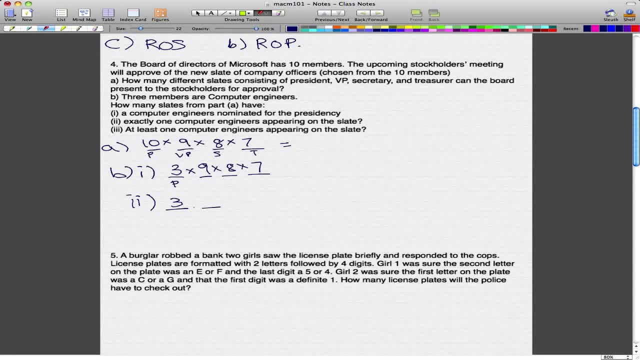 So then, this is three times times seven times six times five. Now this is a little awkward. this is a little different from what we had for I. Why is this seven? Well, it says exactly one computer engineer can be can only appear on the slate, exactly. 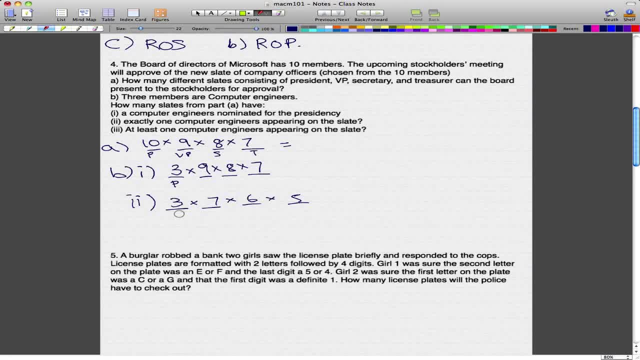 one. So so, using this present rule, one one computer engineer has already been assigned the the position The president role. So then there's already one computer engineer on the slate. So then we cannot have any more engineers on this slate. 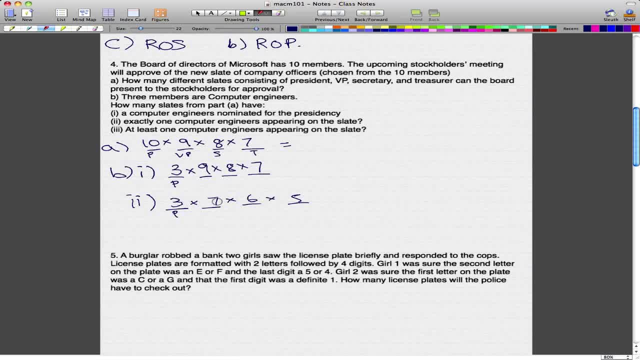 So then, minusing the three from the ten, we have seven people. So, these seven people, one of the seven can be VP, then we are left with six. One of the six can be secretary, and so on. But this is not finished yet. 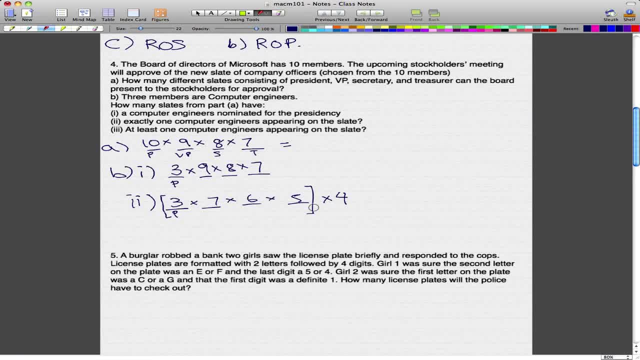 We have four positions, so we have to times it by four to get the correct number, because this is only one case. What if there were? what if? what if a member that was given the president role wasn't a computer engineer and one of the members that are that are computer engineers was given? 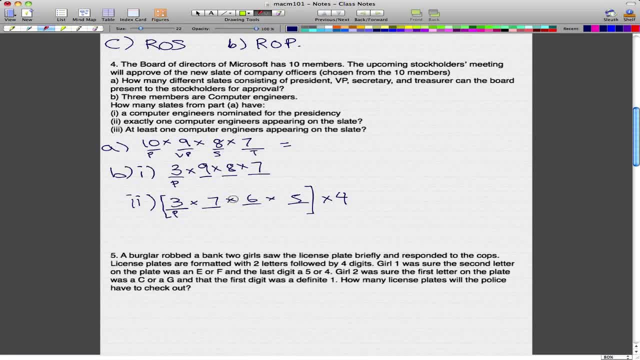 the VP role. So each position is one case. So this is the president president case. There will be another case for VP and there will be another case for treasurer and for secretary. Each in each case, there will exactly be one computer engineer on slate, and that's. 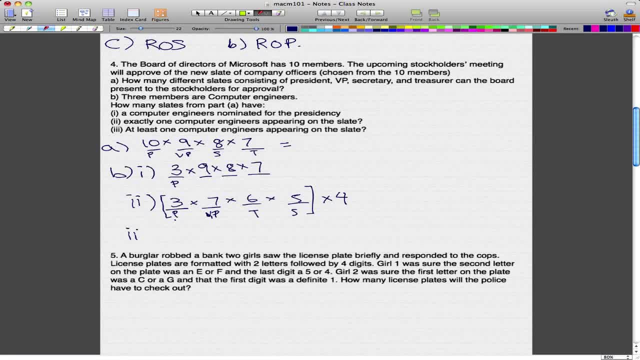 why we times it by four, So number three: at least one computer engineer appears on the slate. Now, this is pretty simple too, So remember that this, this A is pretty much how many different slates consisting of president's, VP, secretary and treasurer can the board present to the stockholders for approval? 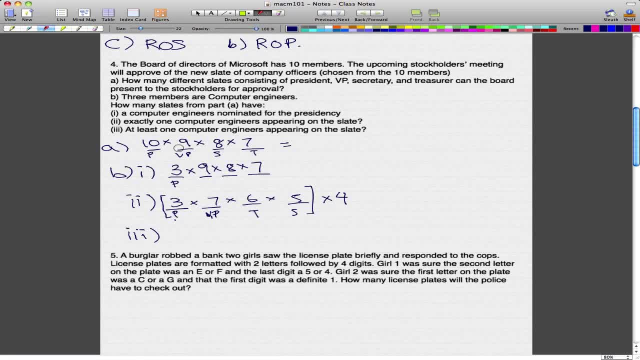 So this incorporates every single possibility that's out there. So we want to take this and the number for this is actually 5,440, and I'm just going to write in these as well. for B, this is 1,512.. Uh, this is 2,520 different ways. 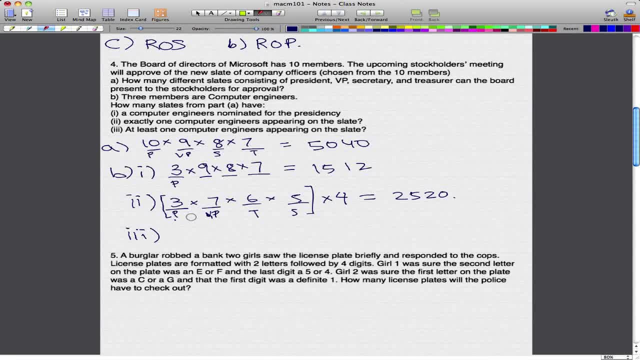 So. So this is the total amount of ways, uh, the total amount of different ways, that, uh, that that members can be elected. So 5,040.. Now we might want to minus that by all the cases where a computer engineer, uh, does. 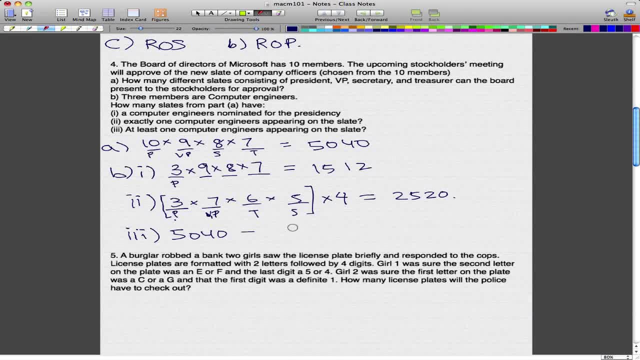 not show up. So that is, uh, that is minus the following: Seven times Six times Five times Four, And that is 820, 840.. So these, this calculation, gives us all the cases, all the different ways in which a computer 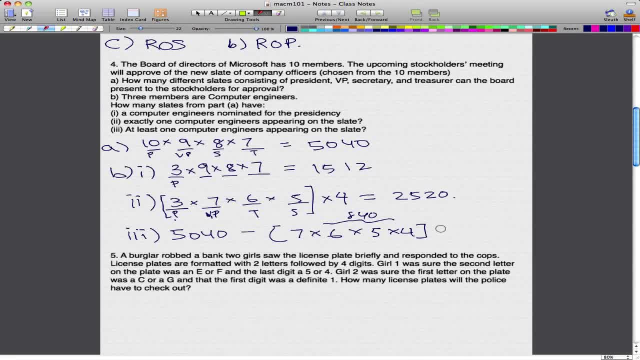 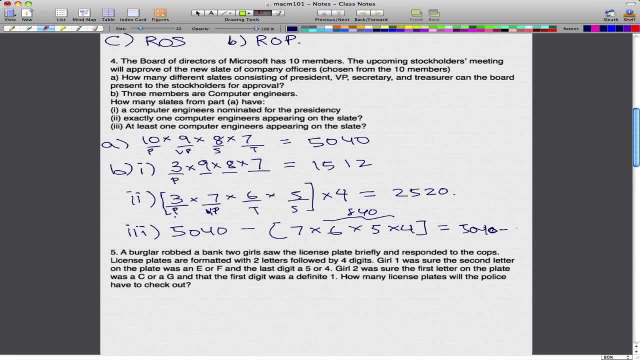 engineer does not appear on the slate. So we take 5,040 minus uh 5,040 minus uh 840, uh, not enough space. Uh 840. Uh 840.. And what we get is we get, uh, we get 4,000 and 4,200 slates. 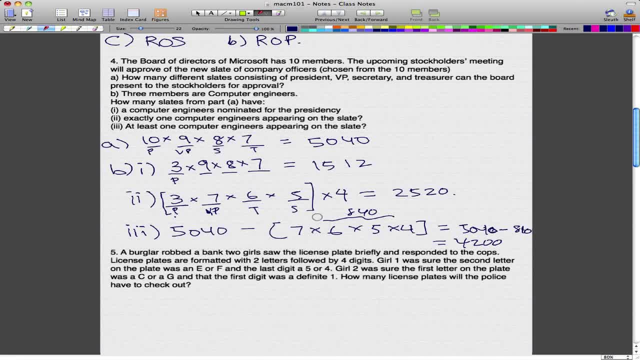 So let me explain this. So at least one computer engineer appears on the slate. If you calculate, if you already have the number for every single possibility that exists, uh, for, for giving positions to these members, and we calculate all the different possibilities. 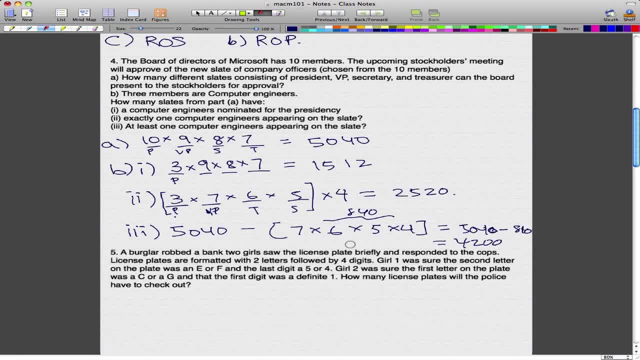 in which, uh, computers, Uh computer engineers, don't appear on the slate, uh, that is, there is no computer engineers on the slate. Then, taking all the different possibilities, minus the possibilities that there are no computer engineers on the slate, gives us the, gives us all the possibilities where there. 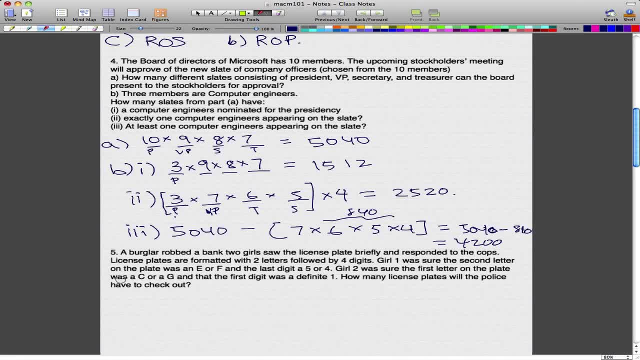 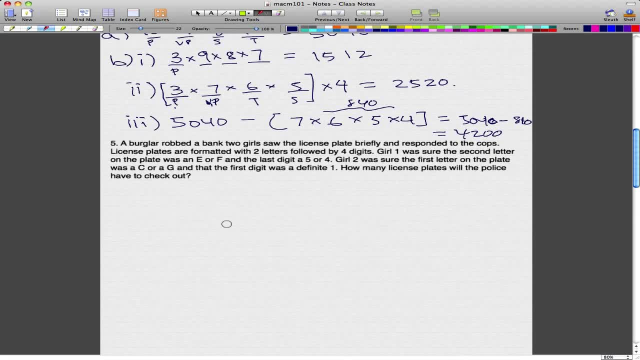 is at least one computer engineers appearing on the slate, And that's uh as simple as I can explain it. I hope you understood that And for this next example, I'll try to go through it as fast as possible because I know. 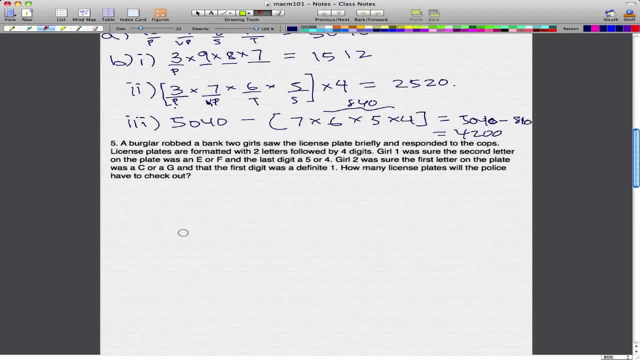 this video is getting Longer and longer by the second. So a burglar robbed, uh, a burglar robbed a bank, and two girls saw the license plate briefly appear and they responded to the cops. Now the license plate is formatted with two letters, uh, followed by four digits.